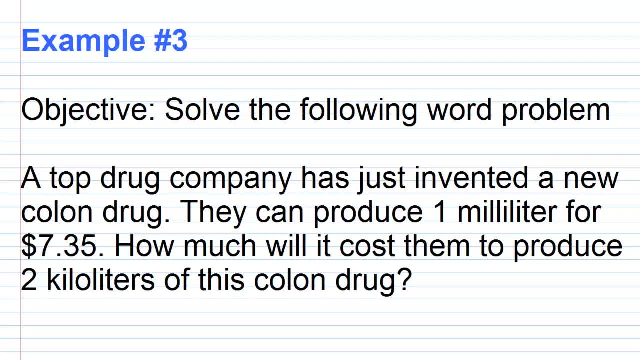 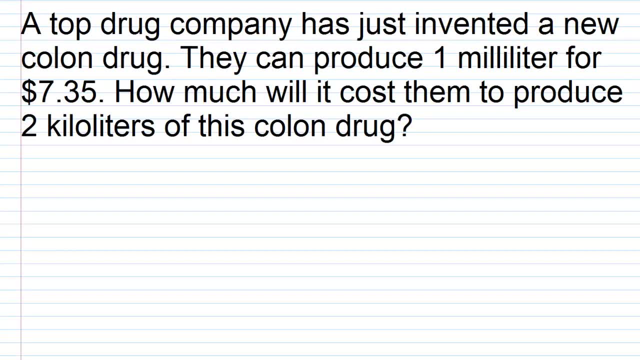 All right, for example three. the objective is to solve the following word problem. So a top drug company has just invented a new colon drug. They can produce one milliliter for $7.35.. How much will it cost them to produce two kiloliters of this colon drug? 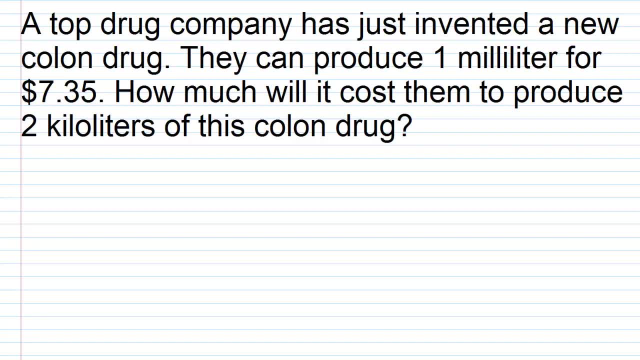 So it's a pretty simple problem here. Just get a little highlighter going And again a top drug company has just invented a new colon drug and they can produce one milliliter. okay, one milliliter for $7.35.. So then our question would be: 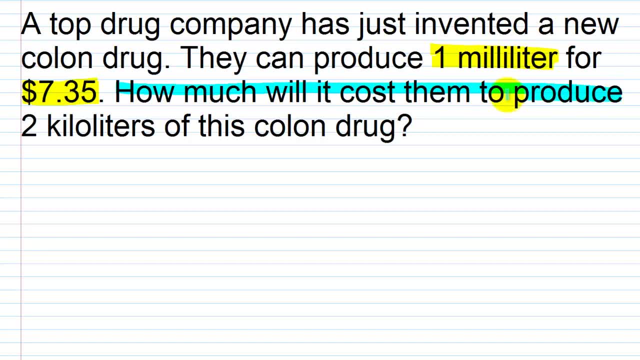 how much will it cost them to produce two kiloliters of this colon drug? Okay, two kiloliters of this colon drug. Pretty simple question again, If they can produce one milliliter of this colon drug, and again for $7.35, and we want to know how much it's going to cost them to produce. 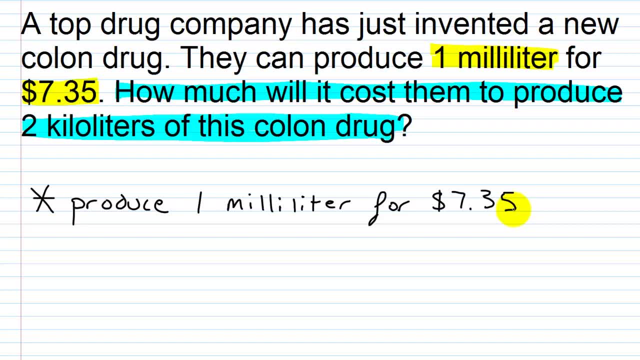 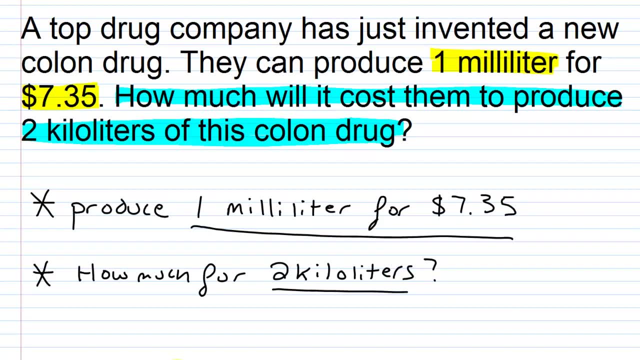 two kiloliters of this colon drug. So how much for two kiloliters? So it's basically a question of how much will it cost them to produce two kiloliters of this colon drug. So basically going to be a two step procedure to solve this And we're going to go from 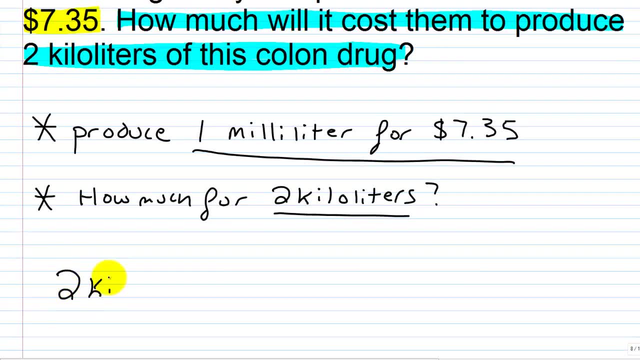 two kiloliters. two kiloliters to an equal amount of milliliters, So we'll put a space here and then milliliters. So how do you convert from two kiloliters to milliliters? Well, we use a prefix chart. So basically we go down to a prefix chart. 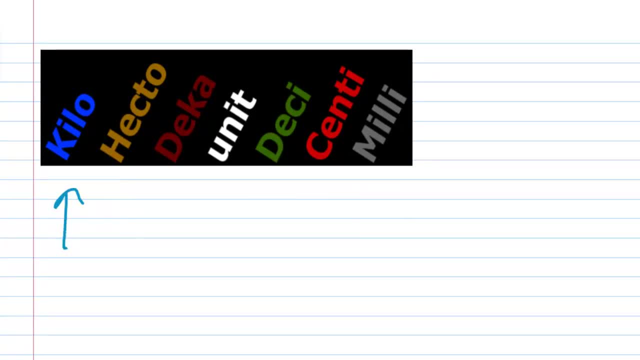 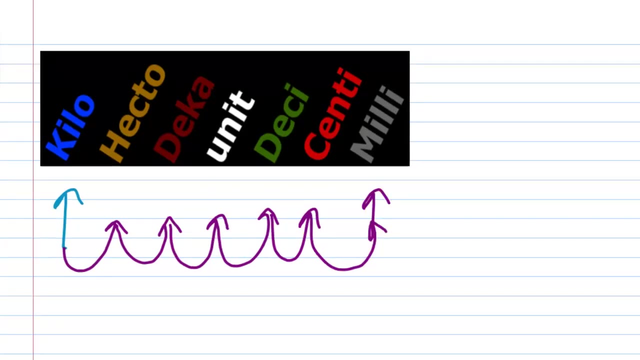 And we find kilo and we find milli. Okay, and we're going to go from kilo to milli. So we're going one, two, three, four, five, six places to the right And so we just max that up here. So we take this number two. 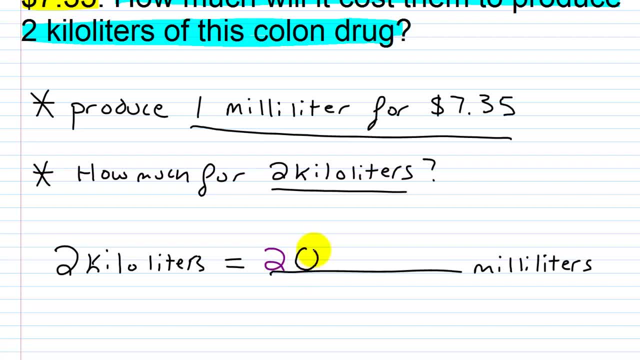 And we just move the decimal six places forward it to the right. So we're going to have to add some zeros here. You're going to want 1,, 2,, 3,, 4,, 5, and then finally 6.. Okay, so you're going to end up with 2 million milliliters is equal to 2 kiloliters. Okay, so now we know that each milliliter costs $7.35.. So all we need to do is multiply 2 million times 7.35.. That's going to give us the cost for 2 kiloliters, So 7.35. 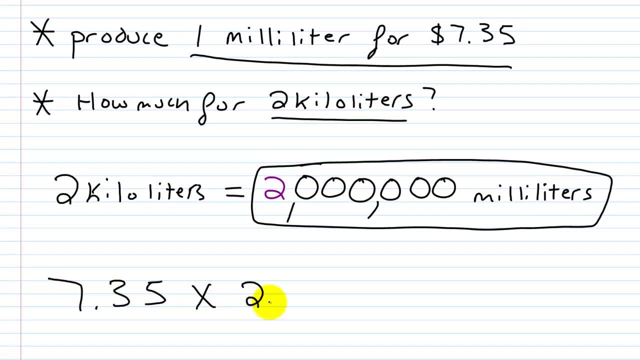 times 2 million. So we can definitely do this without setting up a vertical multiplication. Let's start out by ignoring this decimal here. Pretend we just have 735.. And then we're going to multiply this by 2.. Okay, we're going to use our method where we attach our trailing zeros in the end, So 735. 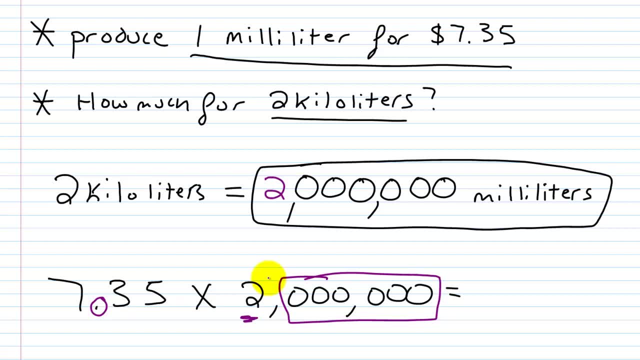 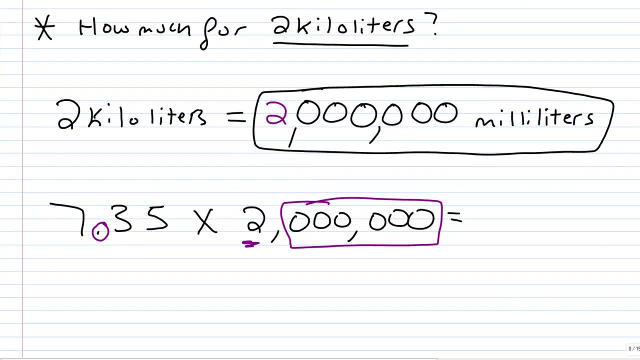 times 2.. Well, 700 times 2 is 1,400.. 35 times 2 is 70. So this would be 1,470 or 1,470.. Now we have 1, 2, 3, 4, 5, 6 trailing zeros. So 1,, 2,, 3, 4, 5, 6, 7, 8, 9, 10,, 11,, 12,, 13,, 14,, 15,, 16,. 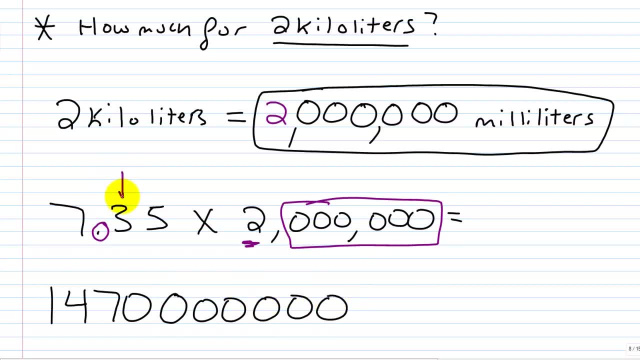 17,, 18,, 19,, 20.. So we have 1,, 2,, 3,, 4,, 5, 6 trailing zeros And then we have 1,, 2 decimal places between the factors. So this is going two places to the left. We'll just erase those zeros there. 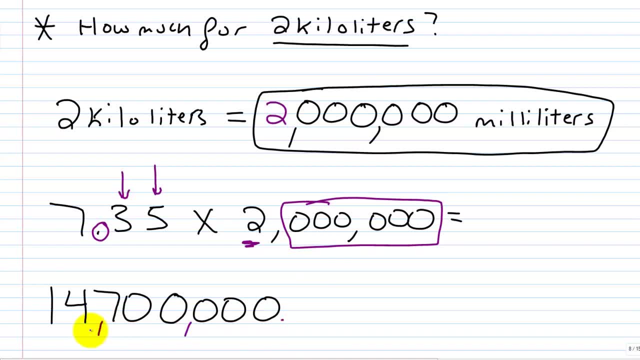 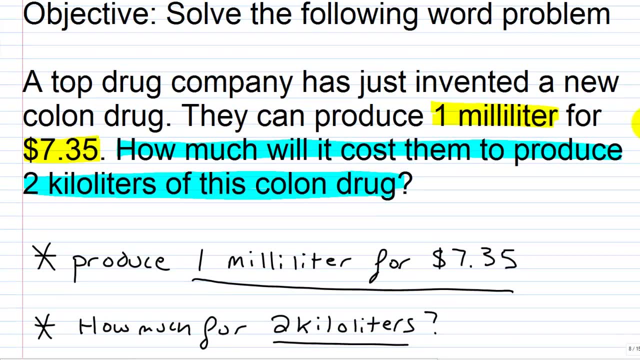 put some commas in and we end up with 14,700,000.. So that's how much it's going to cost for 2 kiloliters of this drug. So how much will it cost them to produce 2 kiloliters of this colon drug? 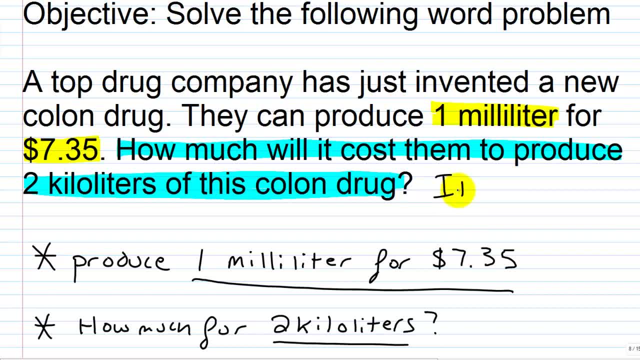 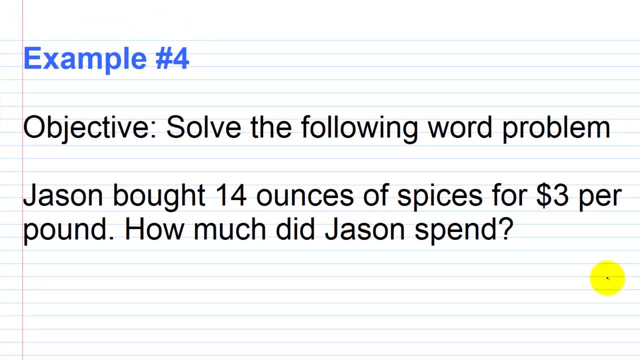 It will cost Fourteen million seven hundred thousand dollars. Okay, for example four. the objective is to solve the following word problem: So Jason bought fourteen ounces of spices for three dollars per pound. How much did Jason spend? So this is a very simple problem. let's get the highlighter going real quick. 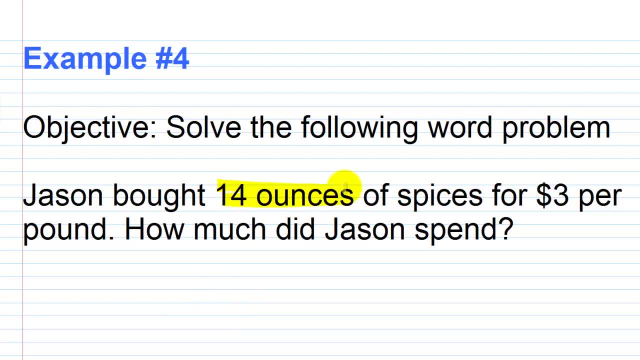 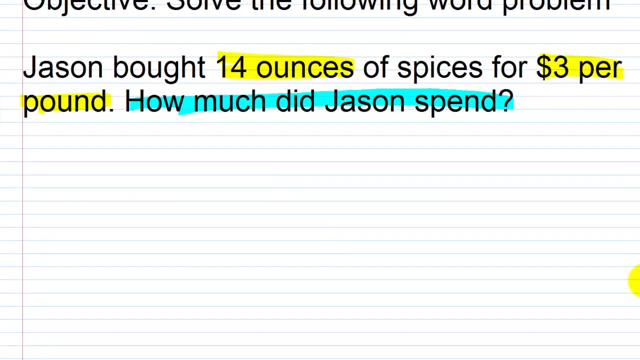 So, again, Jason bought fourteen ounces of spices for three dollars per pound. And then the question: how much did Jason spend? So this is a simple unit conversion problem that we need to set up And basically we need to figure out. well, if Jason bought fourteen ounces of spices, 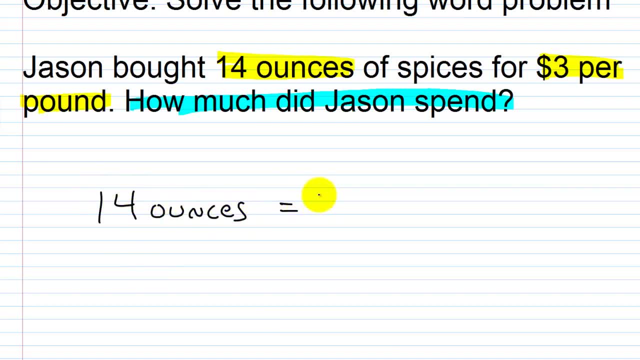 it would equal how many pounds. That's what we need to know, Because we're given the cost in price per pound, right- three dollars per pound. So once we figure out how many pounds we have, we can just multiply this amount by three. 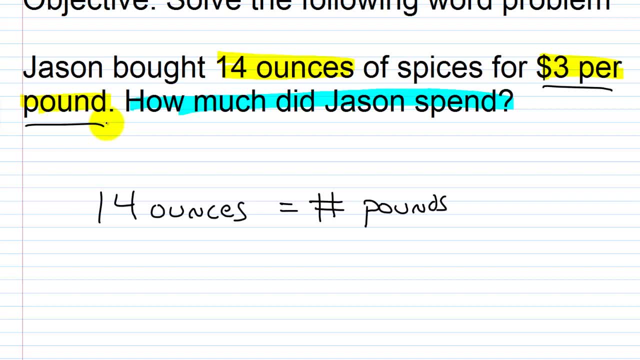 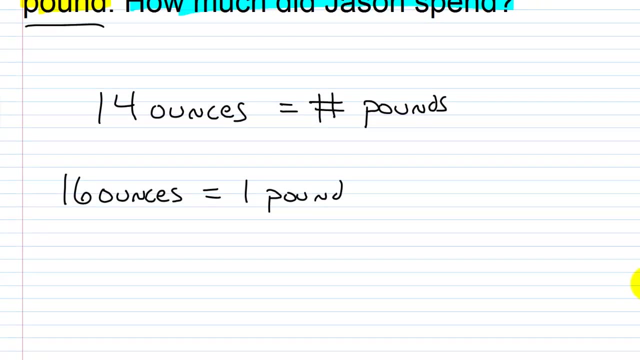 That's going to give us how much Jason spent on these spices. So how many ounces are in a pound? Well, sixteen ounces equals one pound. So to go from ounces to pounds, we have fourteen ounces here. Remember, you want to put the units you want to end up with in the numerator. 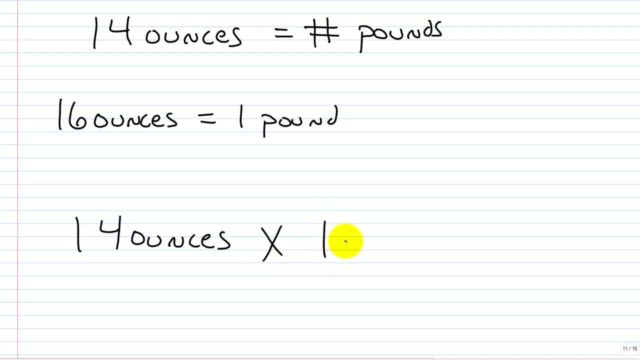 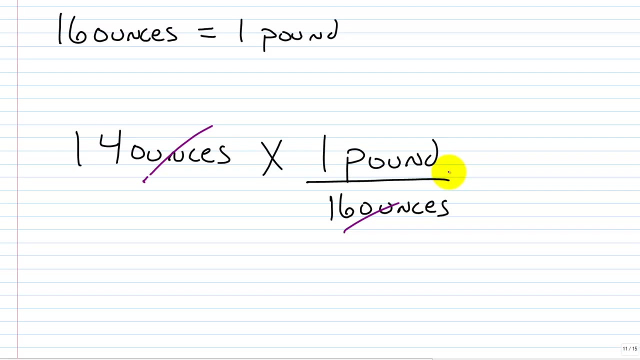 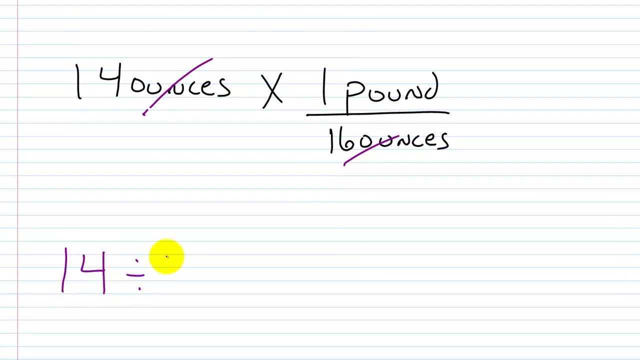 So we want to end up with pounds, so we put one pound in the numerator over sixteen ounces, which is going in the denominator, These units will cancel And we end up with: We end up with fourteen times one pound over sixteen. So we just need to divide fourteen by sixteen and we can figure this out. 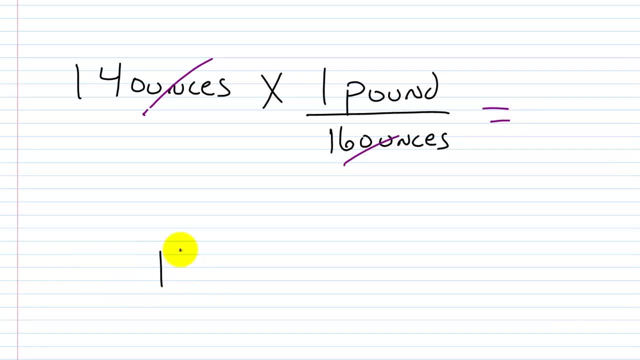 So let's set that up in long division format. so fourteen divided by sixteen. Of course, what you're going to need to do is put a decimal point here, bring that up into the answer and put a zero. So now we have sixteen going into one pound. 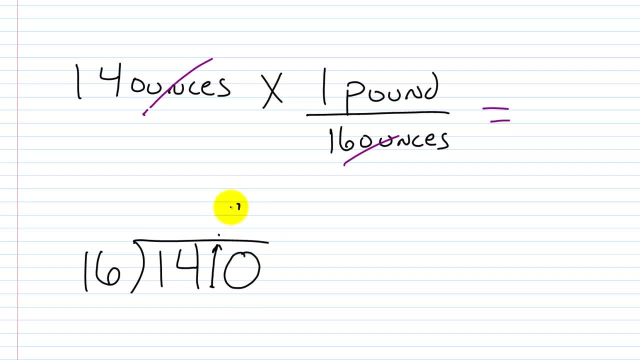 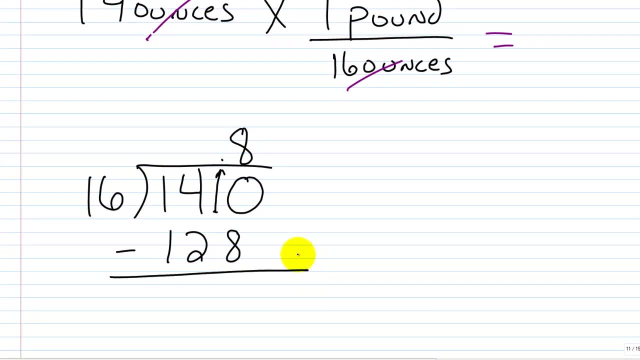 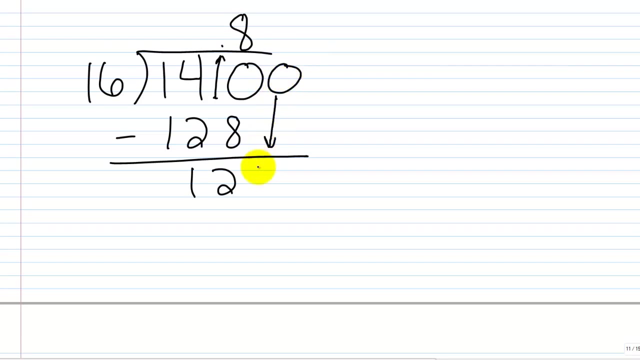 So we're going to do one hundred forty, And that would go in eight times Eight times sixteen is one hundred twenty-eight. We can subtract here and we'll get twelve. What we're going to do is put another zero here. Bring that down. 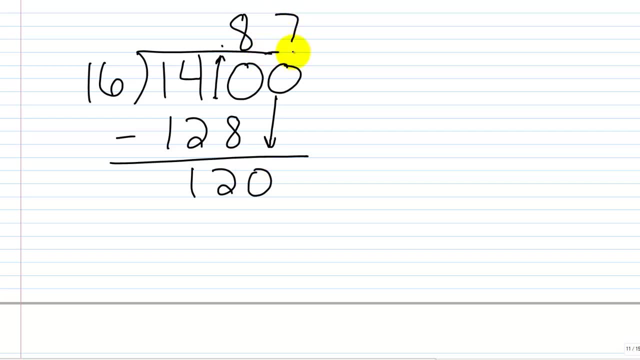 So sixteen would go into one hundred twenty-seven times Seven times sixteen. let's see: seven times ten is seventy. Seven times six is forty-two. So this would be one hundred twelve Subtract, we're going to get eight. Put another zero here, bring that down. 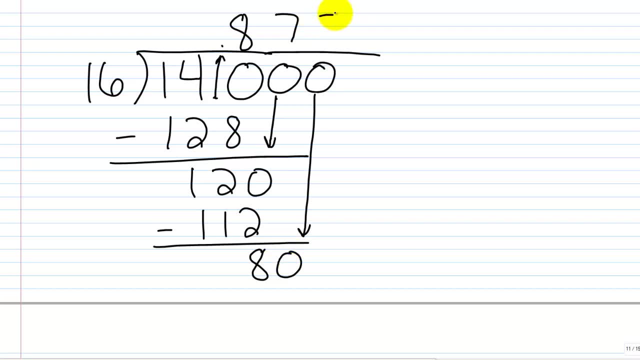 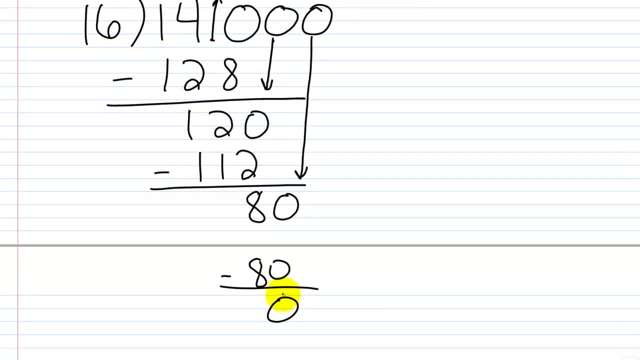 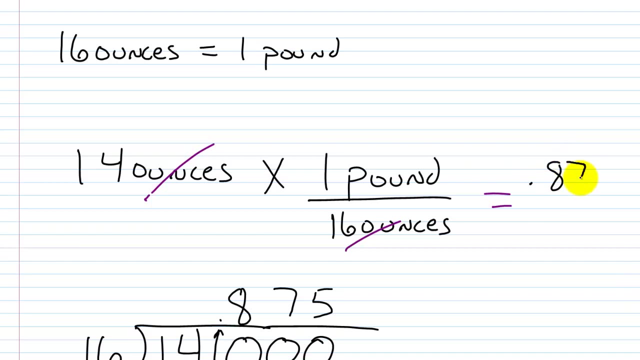 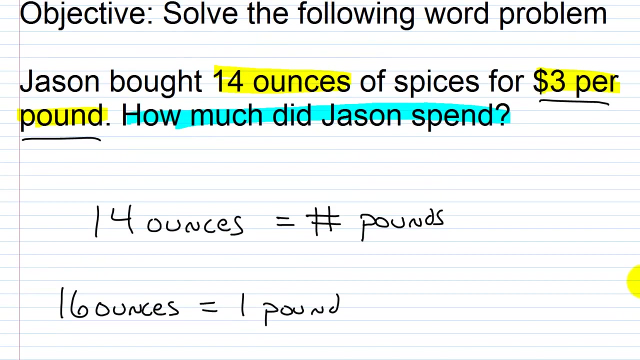 And then sixteen is going to go into eighty, exactly five times. Five times sixteen is eighty Subtract and we get zero. So we end up with point eight seven five pounds. So fourteen ounces is point eight seven five pounds. Okay, Okay. So basically, all we need to do now is multiply this by three dollars, because it's three dollars. 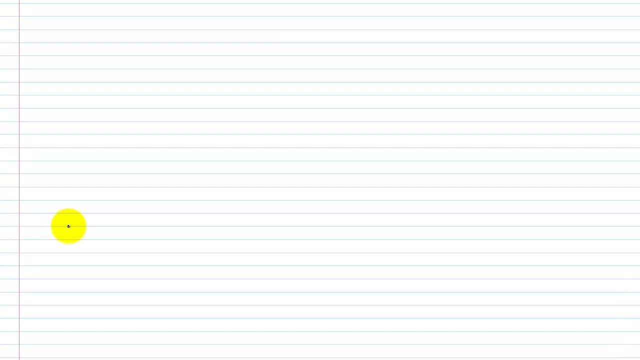 per pound. So we want point eight, seven, five times three. So basically just ignore the decimal and do eight hundred seventy-five times three. Eight hundred times three is twenty-four hundred. Seventy times three is two hundred ten. So twenty-four hundred plus two hundred ten is twenty-six ten. 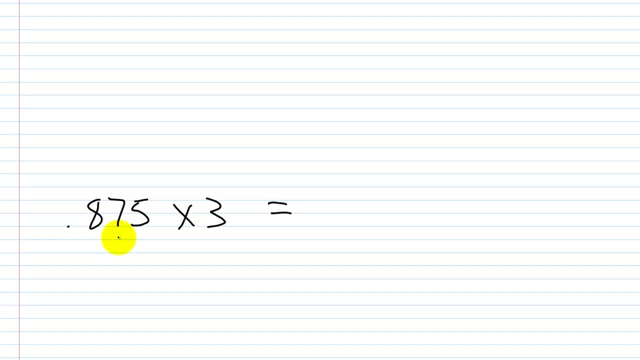 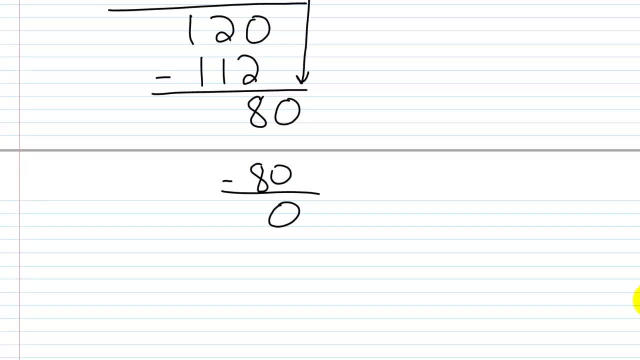 And then three times five is fifteen. So two thousand six hundred ten. Two thousand six hundred ten plus fifteen is two thousand six hundred twenty-five. Then you have three decimal places between the factors. So this is going three places to the left. So we end up with two point six, two, five. 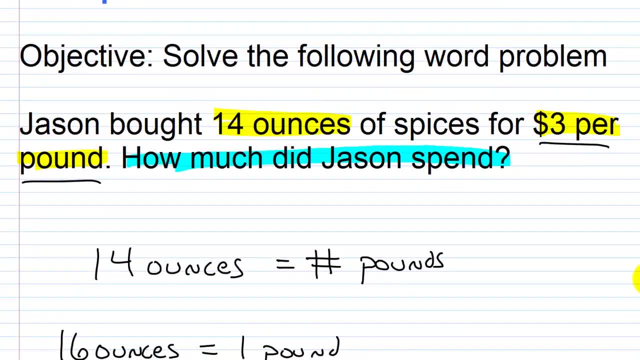 Two point six, two five. And in terms of the problem, how much did Jason spend? Well, he spent Two point six, two five. Two point six, two five. We say two point six, two five, So two point six, If we have two, five here. you have to think about this in terms of money. 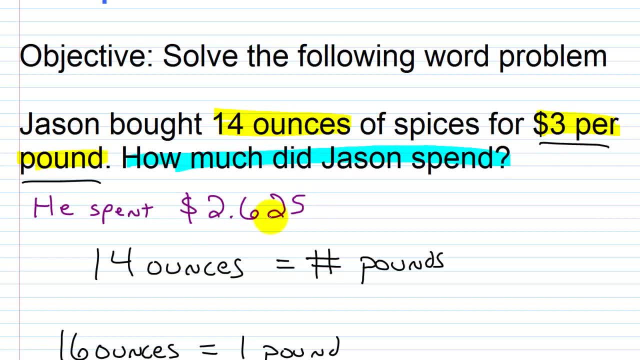 If this was two, five really, you'd have two dollars and sixty-two cents. You can't really have a half of a cent. So we would just round that up and just say two dollars and sixty-three cents. Okay, We would just round that up. 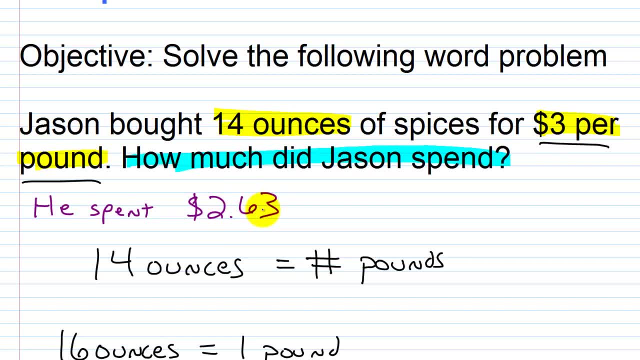 Okay, It's just very close. So it's not exactly two point six, three, But again it's very close. So we're just going to use that answer And to check this again. Jason bought fourteen ounces of spices for three dollars per pound. 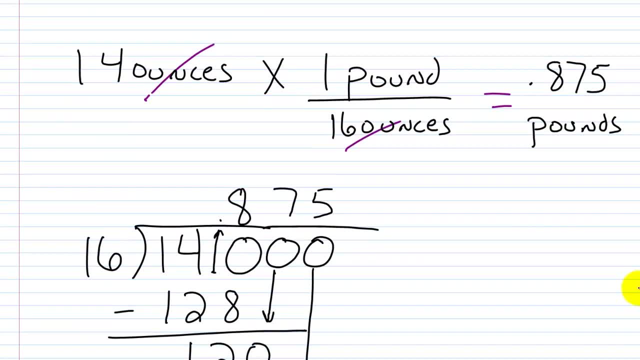 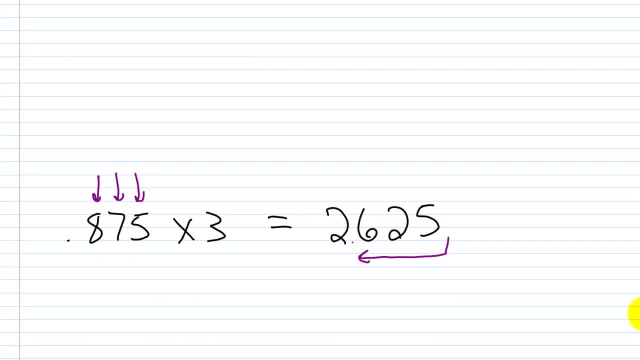 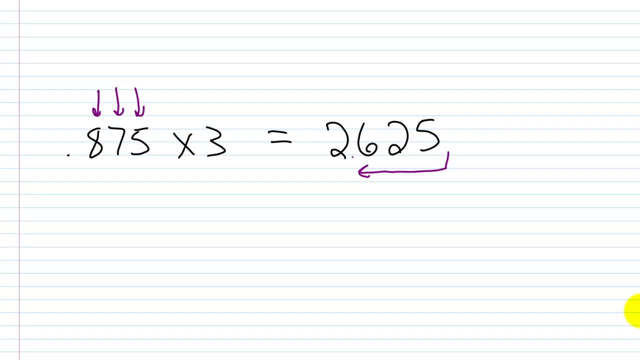 So first we convert fourteen ounces into an equivalent amount of pounds. So fourteen ounces is equal to point eight, seven, five pounds. Then we multiply that by three. Point eight, seven, five by three is two point six, two, five. But in terms of the problem, because we're dealing with a real world application here,